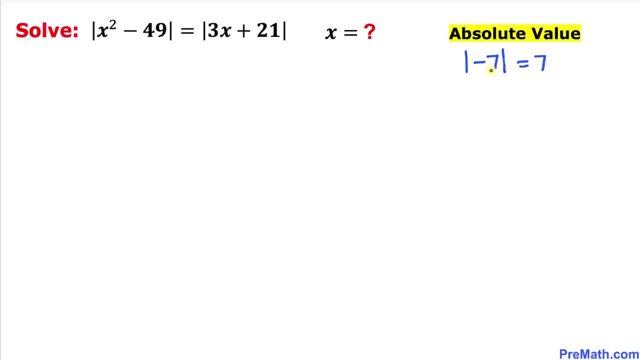 always positive 7, because absolute value means that the distance from zero. how about if i say absolute value of 7, that is going to stay same positive 7 and the absolute value of 0 is going to be simply 0. therefore, in general, we are going to define this: absolute value of x equals to x. 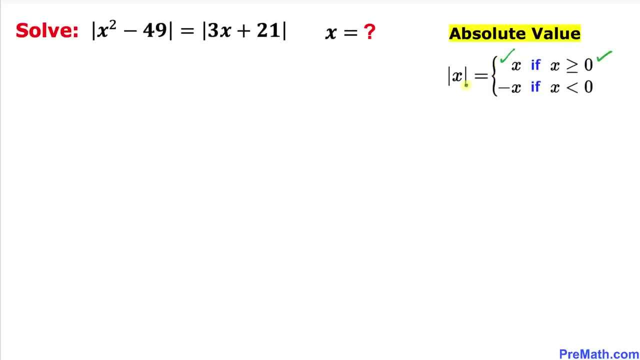 if x is greater than or equal to 0, and this absolute value of x is going to be negative. x less than 0. and now let's focus on this part: x square minus 49. and here I have copied it down. let's focus on this: 49. 49 could be written as a 7 square, so 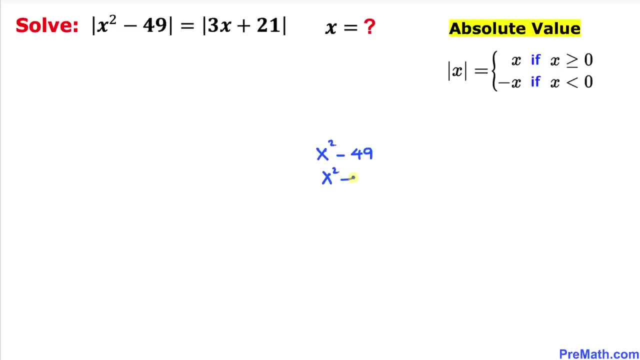 therefore, we can write this one as x square minus 7 square, and now we can see that this represents the difference of two squares. now let's go ahead and use this famous identity: a square minus b square. so therefore this could be written as x minus 7 times x plus 7. so therefore, the left-hand side of this equation. 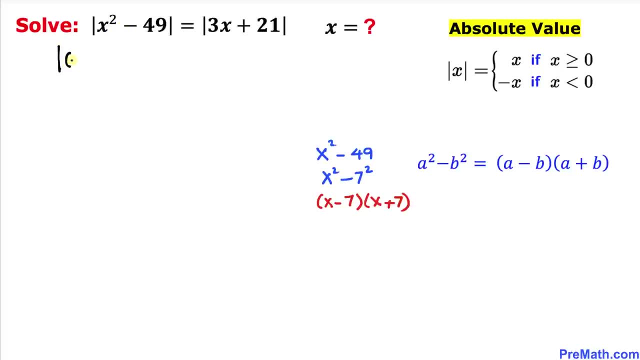 could be written as: the absolute value of x plus 7 times x minus 7 equals to: and here on the right hand side, a 3 is in common, so I can write the absolute value of 3 times a x plus 7 in the absolute value. and now let's go ahead. 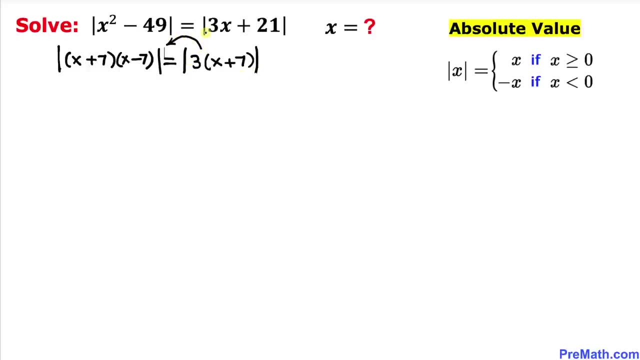 and move this absolute value on the left-hand side, so we can write this whole thing: the absolute value of X plus 7 times the absolute value of X minus 7, and this becomes minus the absolute value three times x plus seven and we have a zero now on the right hand side and here: 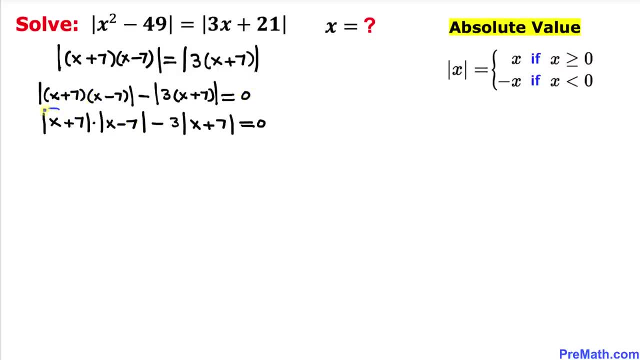 in this next step, I have broken down this absolute value into two individual absolute value and put a times inside and then over. in the next one I brought three outside and now we can see that this absolute value of x plus seven and this absolute value of x plus seven, they are in. 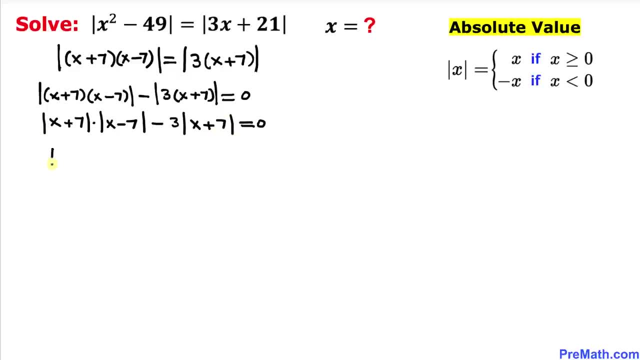 common, so we can factor them out. so let's go ahead and factor that x plus seven, the absolute value outside and inside the bracket, we're going to have the absolute value of x minus seven, and then minus three equals to zero. now we can see. we have our two factors. 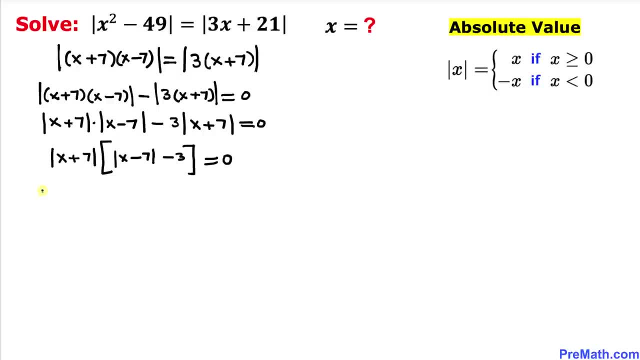 equal to zero, zero. let's go ahead and separate them. i can write the first one, absolute value of x plus 7 equals to 0, or the other one. i'm going to write down the absolute value of x minus 7 and then minus 3. 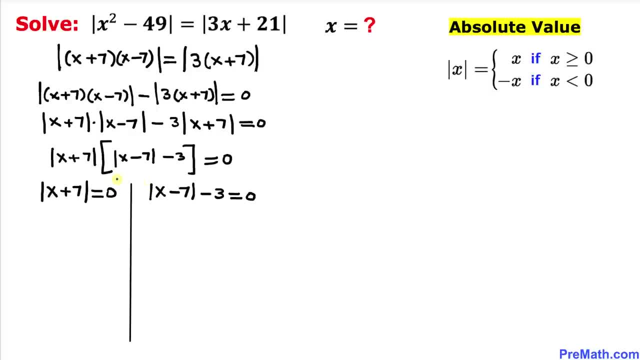 equals to 0.. now let's focus on this absolute value of x plus 7, equal to 0. so that means our x plus 7 value is going to be 0. so that means x value turns out to be simply negative: 7. and now? 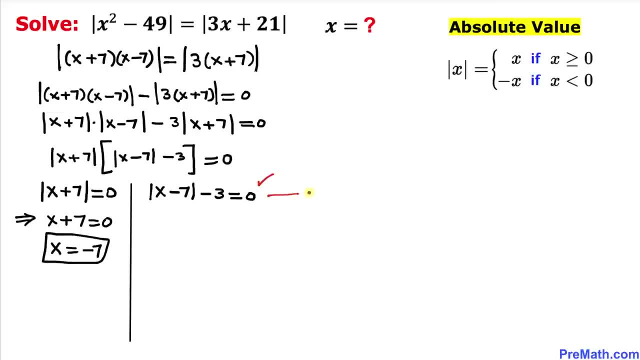 let's focus on this equation, let me go ahead and call this as an equation number one. and now let's go ahead and apply this absolute value definition on this part: x minus 7, when x is greater than or equal to 0. therefore, in case 1, i'm going to say if this x minus 7 is greater than or equal to 0. 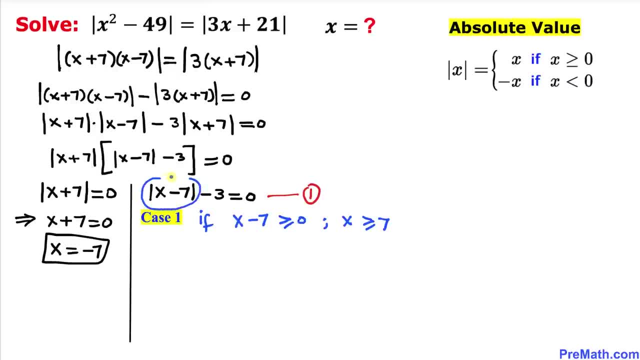 so therefore, this absolute value of x minus 7 could be written as: the absolute value of x minus 7 equals to positive x minus 7. therefore, our this equation 1 is greater than or equal to 0. so therefore, our x plus 7 is greater than or equal to 0. so therefore, this is going to become: 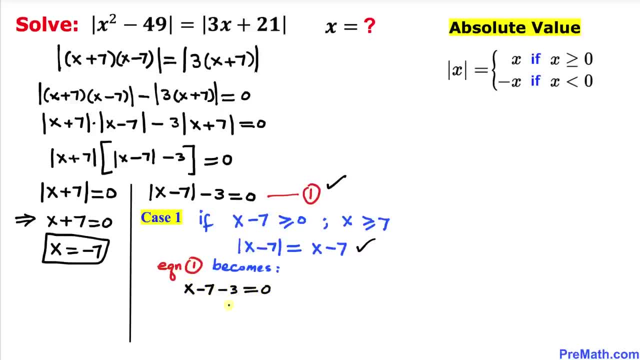 when we apply this definition, this is going to become x minus 7 and minus 3 equal to 0. let's combine the like terms so this become x minus 10 equal to 0. that means x value turns out to be simply positive 10.. 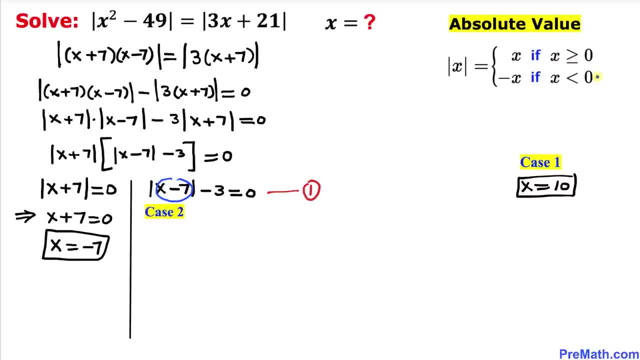 And we are going to consider this second case- when x is less than 0. Therefore, in this second case I can write: if this x minus 7 is less than 0. So that means our this absolute of x minus 7 is going to be equal to negative times x minus 7, which is same as negative x, and then this become plus 7.. 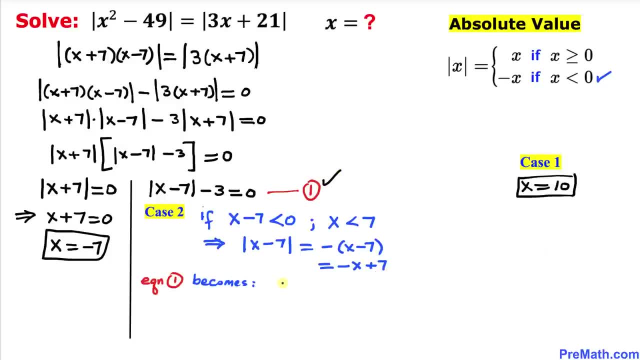 So, therefore, our this equation 1 is going to simply become negative x plus 7.. And then Minus 3 equals to 0. Therefore, our x value turns out to be simply positive 4.. And here's our final step. 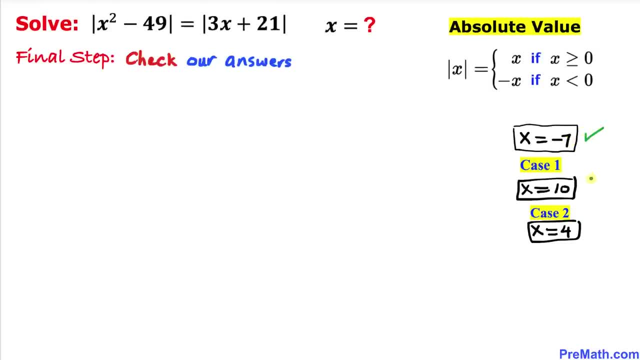 Let's go ahead and check all of these three solutions: x equal to negative 7,, x equal to 10, and x equal to 4.. Now let's go ahead and check our solution: x equal to negative 7.. That means, wherever we see x, I am going to replace it. 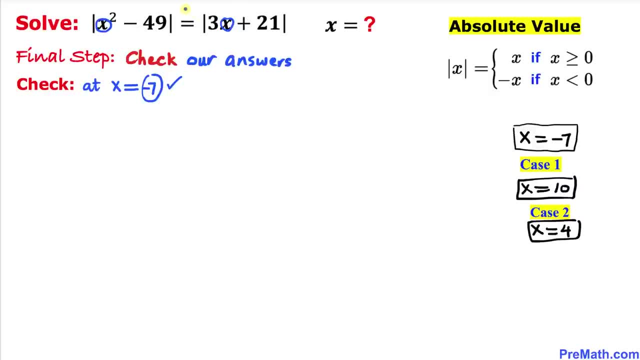 And by negative 7 and see if the left hand side is equal to right hand side. And here we plugged it in and we can see that 0 turns out to be equal to 0. And this, indeed, is a true statement. So, therefore, we are going to conclude that this, indeed, is x equal to negative 7 is our solution. 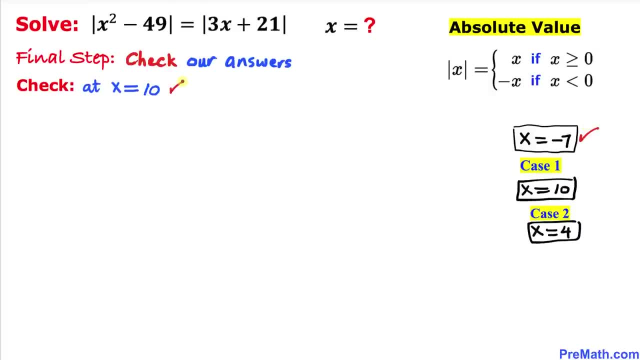 And now let's go ahead and check our solution at x equal to 10.. And here I plugged in This x equal to 10 value And we can see that the left hand side is 51 and the right hand side is 51 as well. 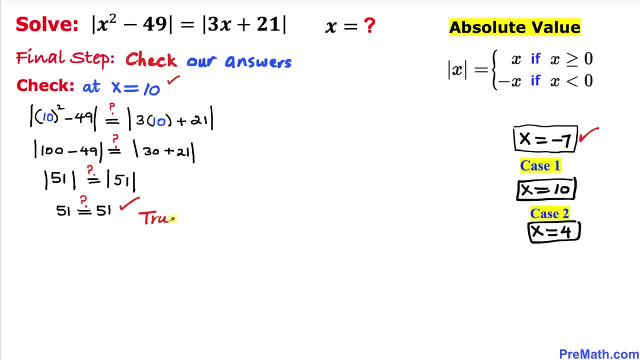 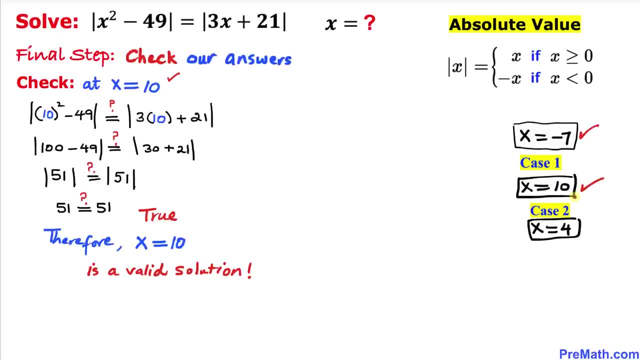 So we can see that this is indeed a true statement. So, therefore, we conclude that x equals to 10 is our valid solution as well. And now, finally, let's check the solution at x equal to 4.. And here we applied x equal to 4 and we can see that 33 turns out to be equal to 33..